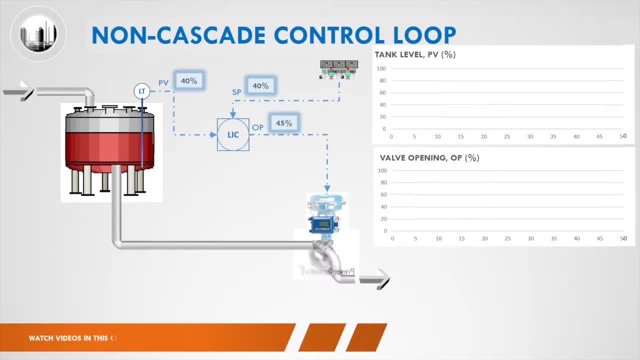 disturbance, for example, this case, the increase of downstream back pressure. Since the large size of the tank causes a very large process lag, the tank level will increase only after a long period of time. The level transmitter will sense the new PV Due to difference between the PV and set point, the output, which is the command, to the control. 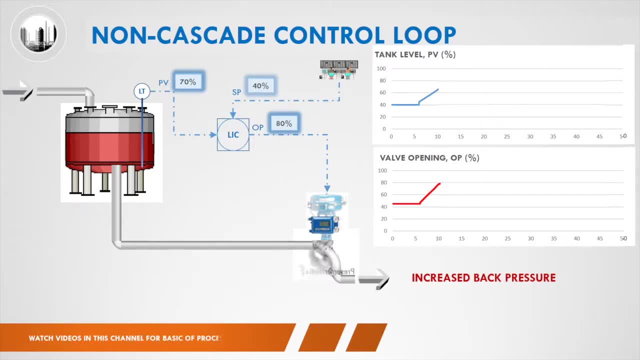 valve will increase. This will cause the tank level to reduce back to the set point. Also, the tank level is now returned back to the set point. There is a large overshoot of the PV due to the process lag. If this large overshoot is not acceptable, cascade. 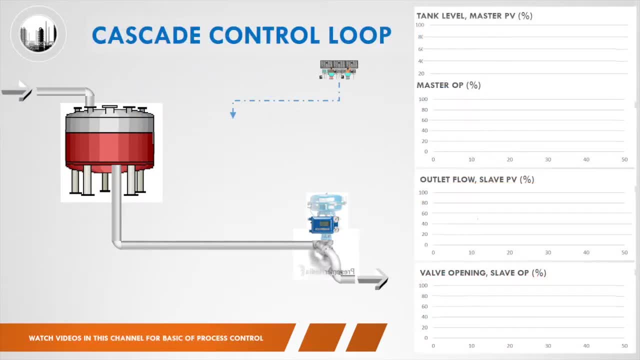 control can be applied. Cascade control consists 2 control loops. The first control loop is the master control loop. The second control loop is the slave control loop. The output of the master control loop is the set point of the slave control loop In this cascade control loop. 2- PV, which is the level and flow control. 1- output, which is the control valve. 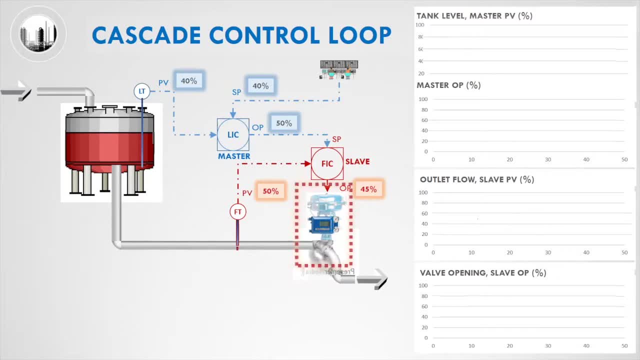 Let us evaluate the same scenario. when the pressure downstream increases Immediately after the back pressure occurs, the outlet flow will immediately reduces Due to the difference between the flow, PV and set point. the output will increase After the control valve opens more. the outlet flow will increase back to the set point. 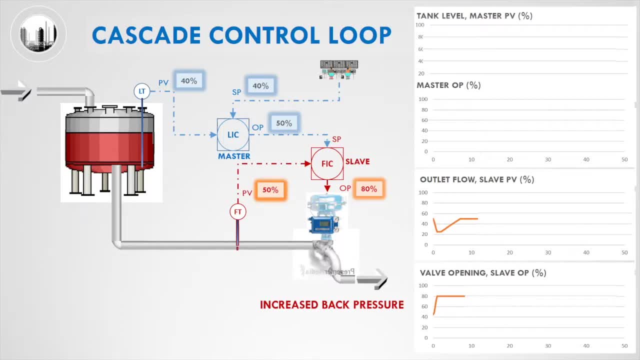 This example demonstrate the advantage of cascade control over normal closed loop. Cascade control allow faster correction of error due to disturbances. Let us evaluate what will happen when the level increase. The level transmitter will sense the increase of the level Due to the difference between the level PV and set point. 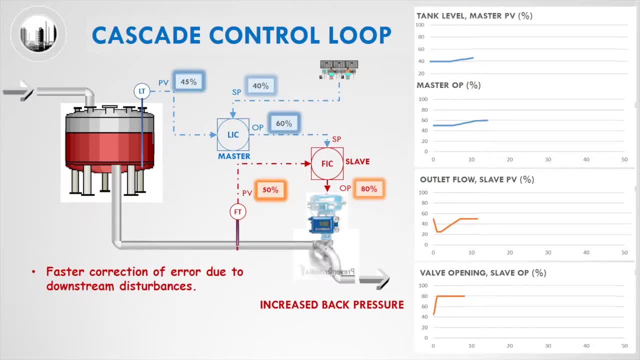 the output of the level controller will increase. This will cascade to the increase of flow controller set point. Due to the difference between the flow PV and set point, the output of the flow controller will increase. This will cause the control valve to open more. 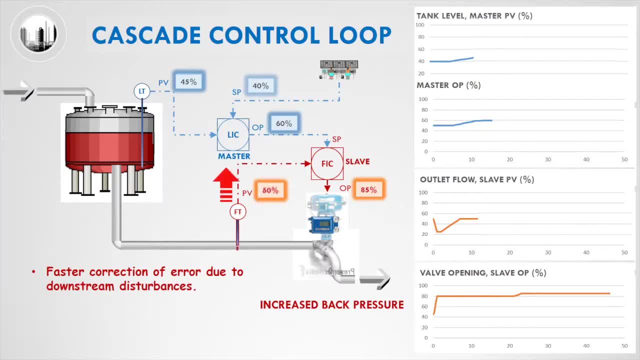 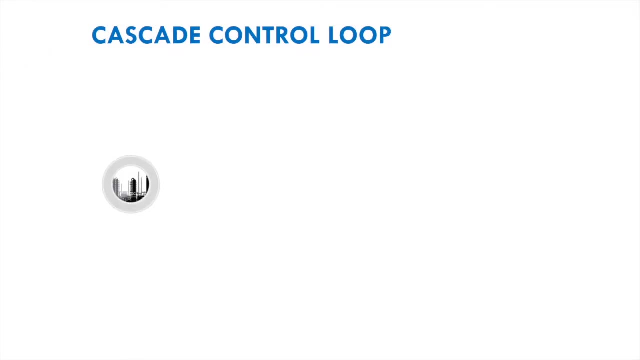 Thus the tank level will reduce back to the set point. We have completed the topic of cascade control. There are more videos in this channel related to process control. Please feel free to watch. Thank you for watching.